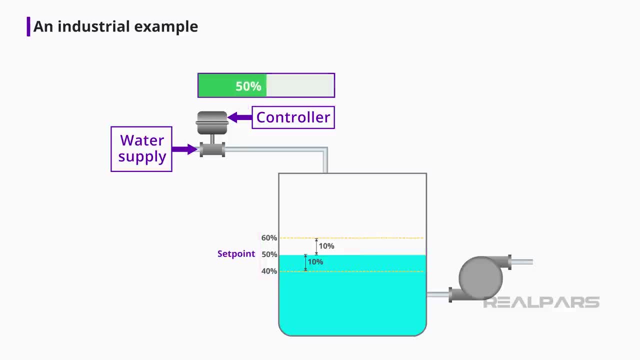 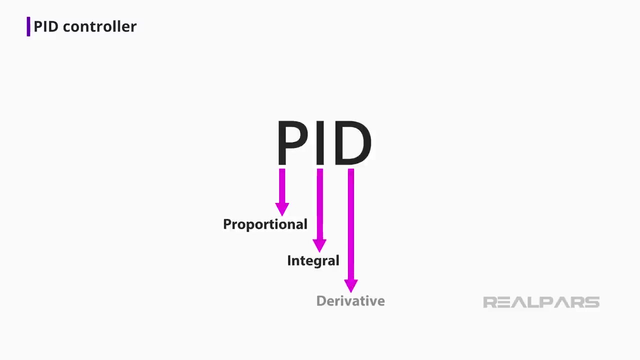 Okay, well what if it's possible to throttle the valve and place it in any position between on and off? Now we can move on to talking about a PID controller. P stands for proportional, I stands for integral and D stands for derivative. 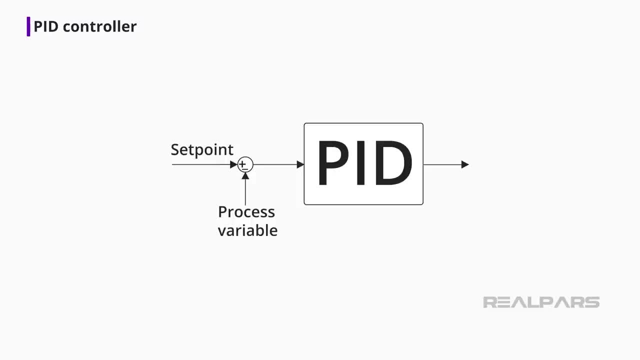 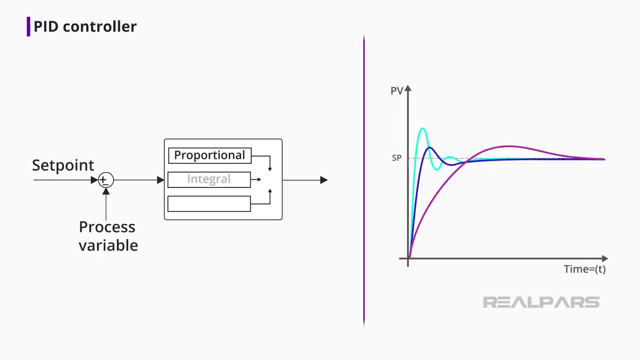 Because every process responds differently. the PID controller determines how much and how quickly correction is applied by using varying amounts of proportional, integral and derivative action. Each block contributes a unique signal that is added together to create the controller output signal. Let's look at how a PID controller fits into a feed. 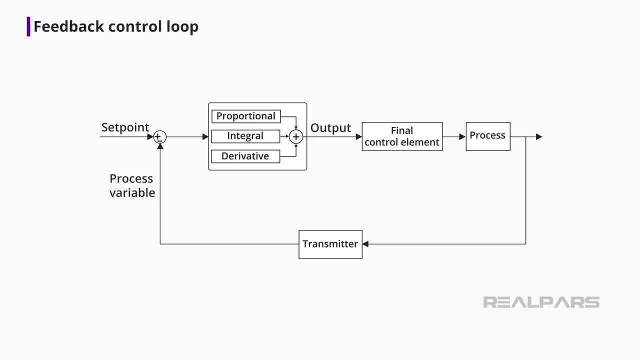 back control loop. The controller is responsible for ensuring that the process remains as close to the desired value as possible, regardless of various disruptions. The controller compares the transmitter process variable or PV signal and the setpoint. Based on that comparison, the controller produces an output signal. 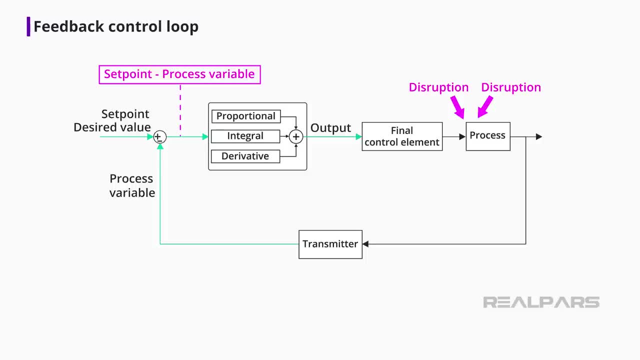 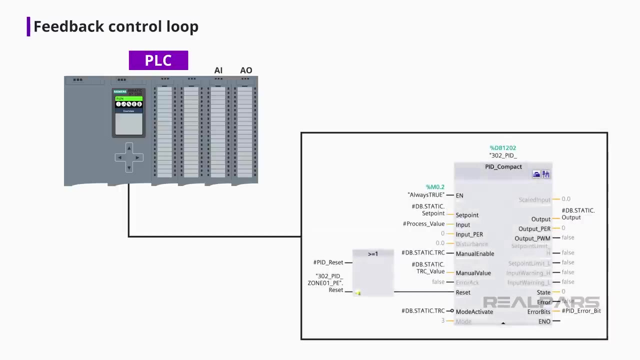 to operate the final control element. This PID controller output is capable of operating the final control element over its entire 100% range. Most modern PID controllers are part of a PLC or DCS and are created in the program control logic using block commands. 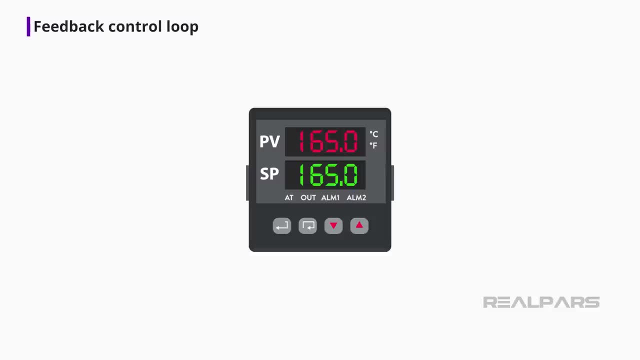 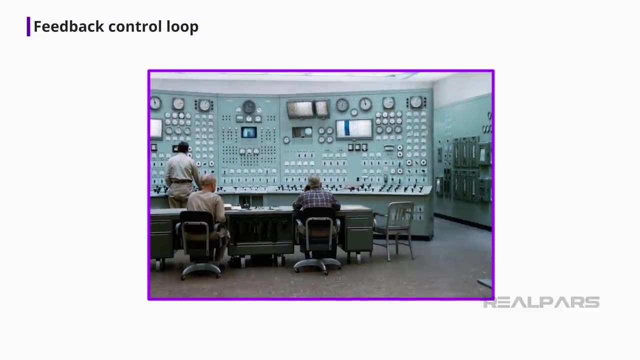 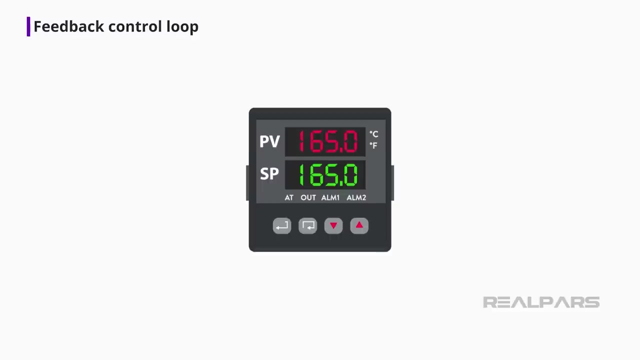 Before PLCs came along, a PID controller was a stand-alone device responsible for controlling one loop. A control room would have dozens or hundreds of stand-alone controllers mounted on a panel. There are still many stand-alone PID controllers being manufactured and used today. 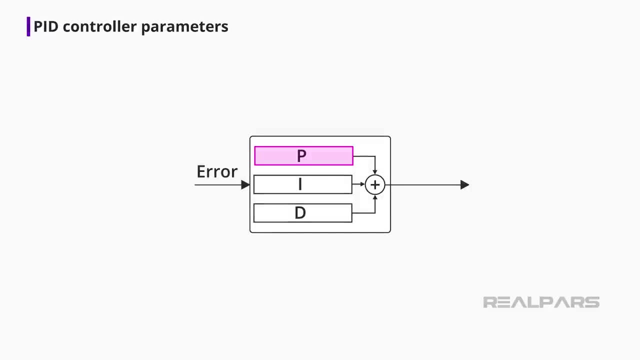 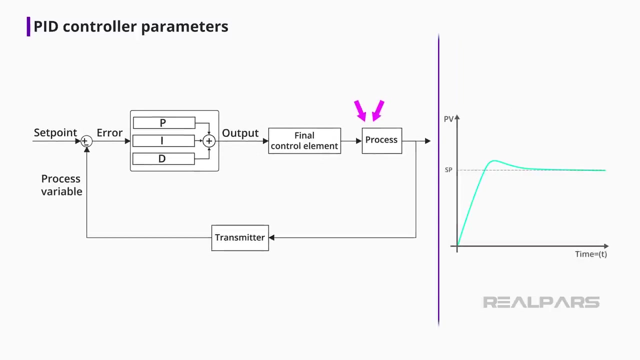 Ok, let's get back and talk about what each of the P, I and D components of the PID controller does. Remember, earlier we said that the PID controller is responsible for ensuring that the process remains as close to the setpoint as possible, regardless of various disruptions. 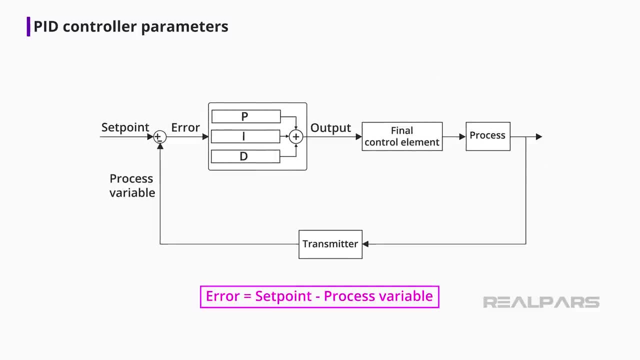 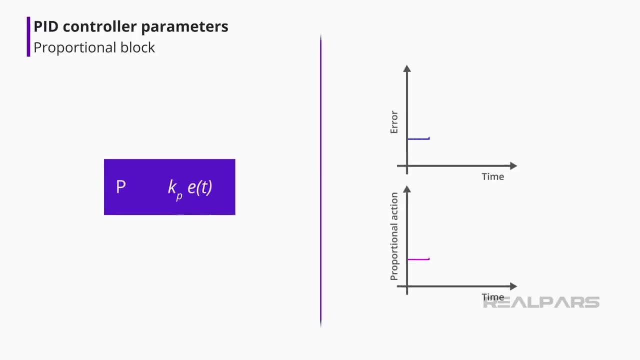 Let's refer to the difference between the process variable and the setpoint as the error signal. The proportional block creates an output signal proportional to the magnitude of the error signal. Unfortunately, the closer you get to the setpoint, the less it pushes. 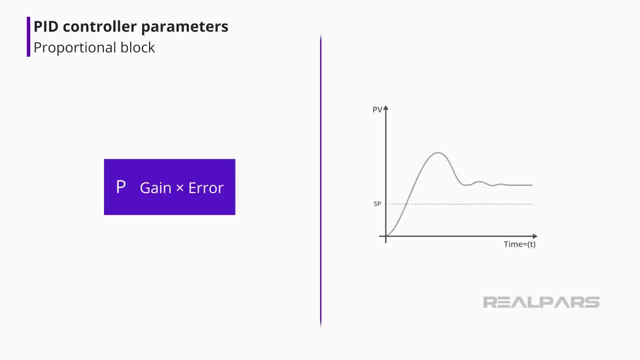 Eventually, the process just runs continuously close to the setpoint, but not quite there. That's when integral jumps in. The integral block creates an output proportional to the duration and magnitude of the error signal. The longer the error and the greater the amount, the larger the integral output. 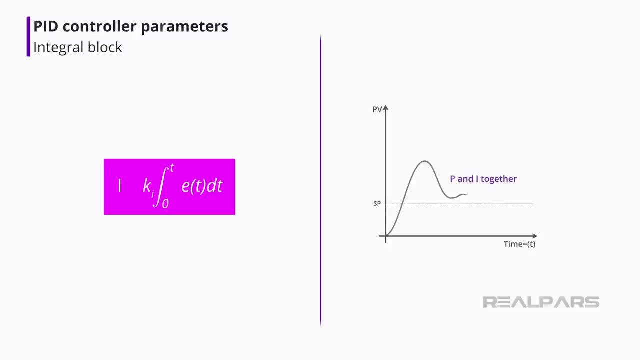 As long as an error exists, integral action will continue. The derivative block creates an output signal proportional to the rate of change of the error signal. The faster the error changes, the larger the derivative output. Derivative control looks ahead to see what the error will be in the future and contributes to the control room. 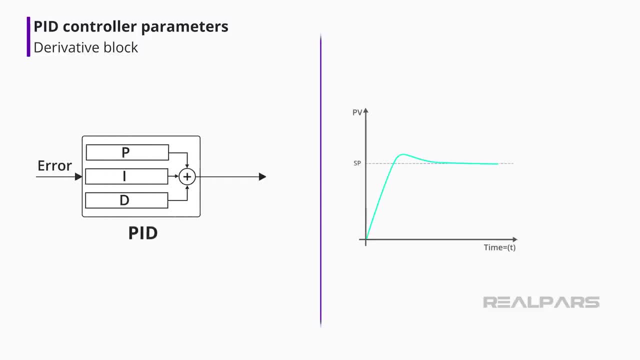 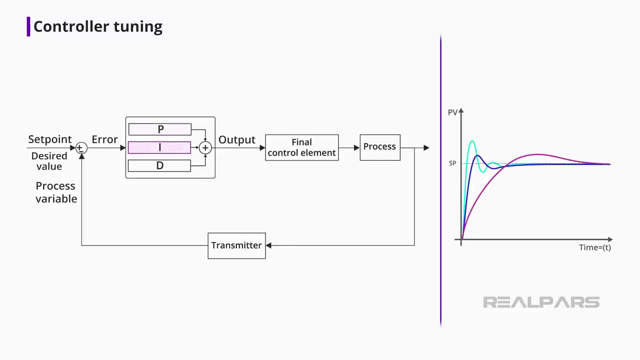 The controller is set to the controller output accordingly. That brings us to a term called controller tuning. We said earlier that every process responds differently and that the PID controller determines how much and how quickly correction is applied by adjusting proportional, integral and derivative action. 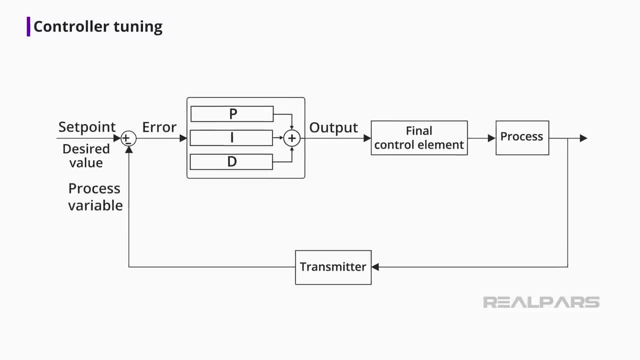 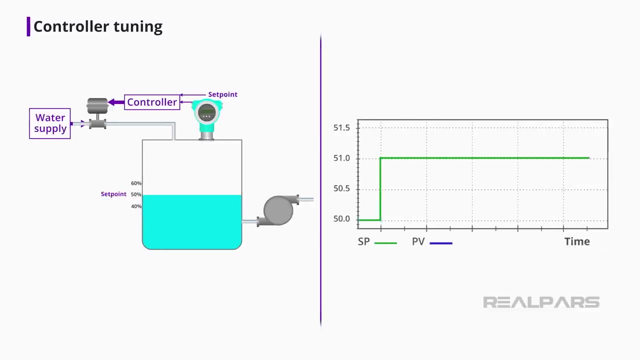 Controller tuning involves correctly setting the controller P, I and D values for specific process requirements. Interestingly, the correct settings achieved by controller tuning can differ vastly between processes because of specific requirements. For example, after the controller has been tuned, a setpoint bump of 1% in a tank-level control produces a quarter-wave damped response. 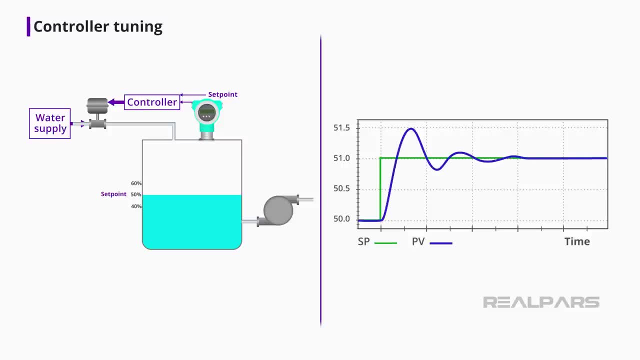 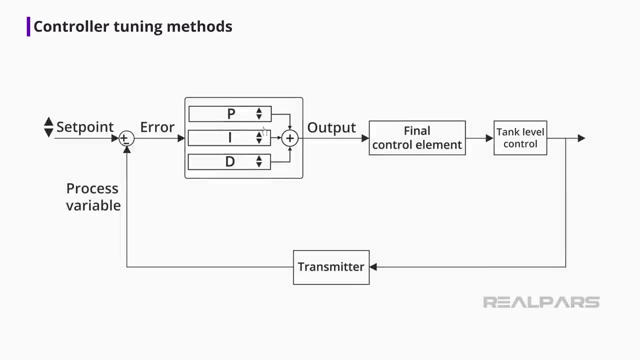 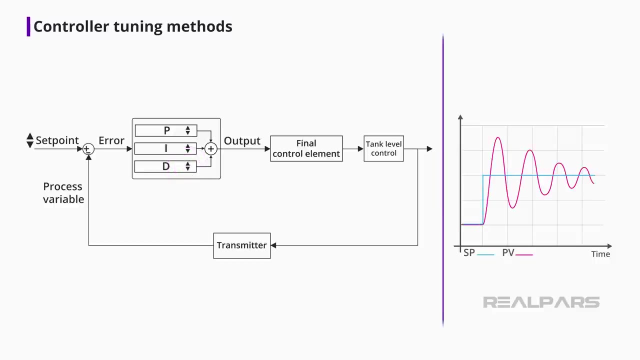 This type of response may be suitable in a tank-level process but could be disastrous in a motion control process. There are many different manual methods for tuning a controller. that involves observing the process response after inflicting controller setpoint changes. One method involves increasing the amount of setpoint change. 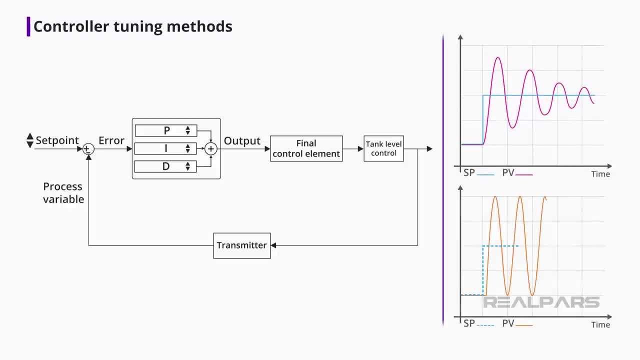 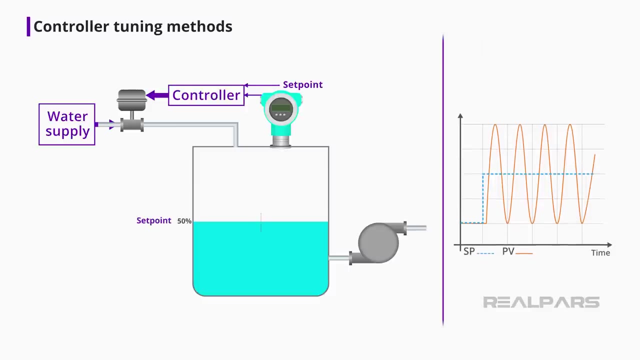 and repeating the procedure until the process enters a state of steady-state oscillation. This method of tuning produces adequate results but is often impractical in many applications. For example, how practical is it to force the fluid level in a large tank to reach a steady-state oscillation? 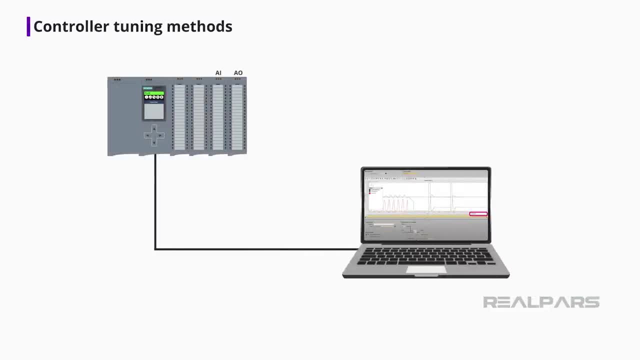 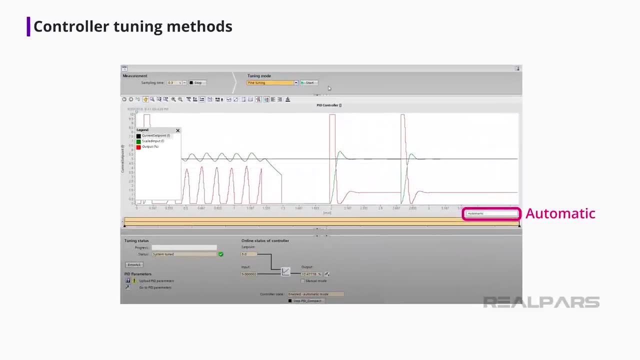 Most process controllers- PLC and DCS loop controllers- sold today have auto-tuning capability. The PID controller learns how the process responds to a change in setpoint and suggested PID settings, Regardless of whether the initial PID parameters are derived from the manual or auto-tuning methods. 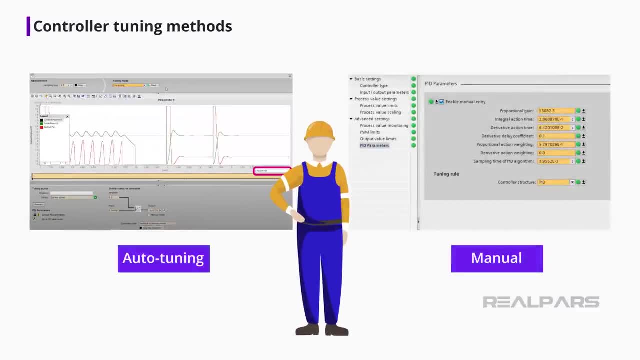 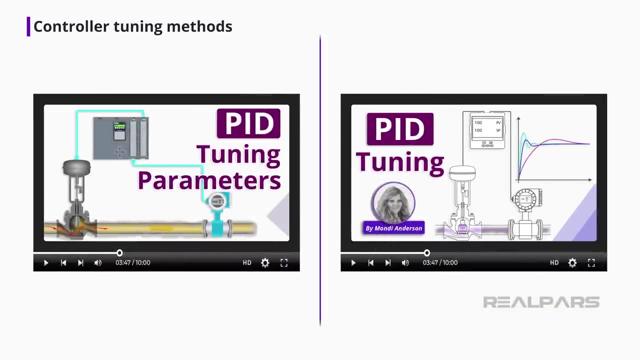 additional tweaking is often required by seasoned automation professionals to get the response desired. That should do it for this video. If you want to learn more about PID control, you might want to watch our other two videos called What are PID Tuning Parameters and How to Tune a PID Controller. 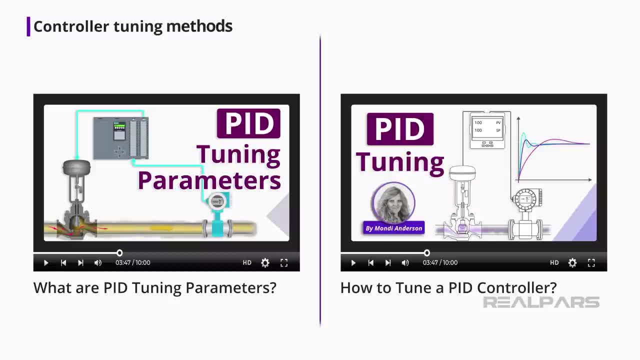 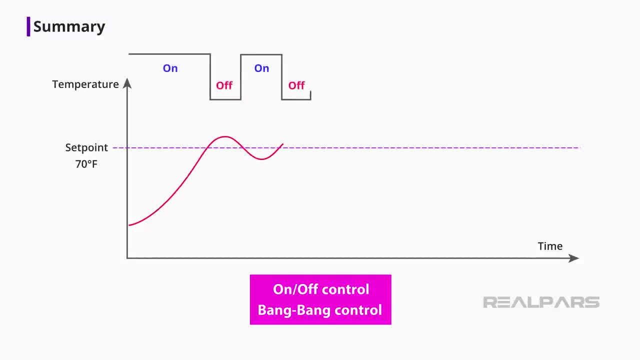 You can find the links to these videos in the description. Ok, let's review. An on-off or bang-bang controller has only two output conditions and switches abruptly between these two conditions. In a PID controller, P stands for Proportional, I stands for Integral and D stands for Derivative. 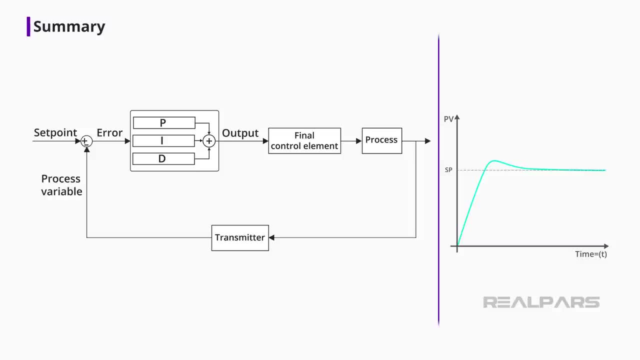 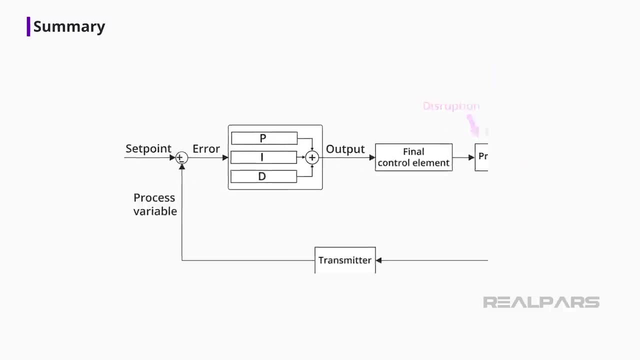 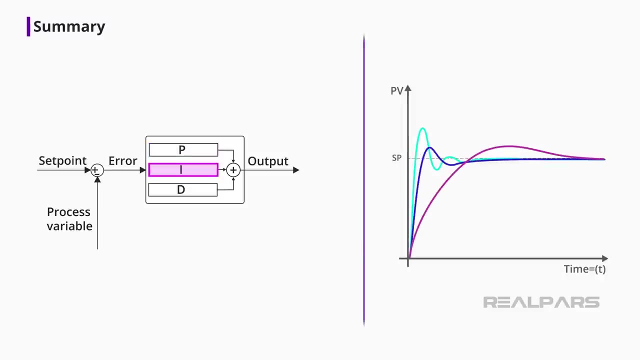 The PID controller is responsible for ensuring that the process remains as close to the desired value as possible, regardless of various disruptions. The PID controller determines how much and how quickly correction is applied by using varying amounts of P, I and D action. The Proportional block creates an output signal. 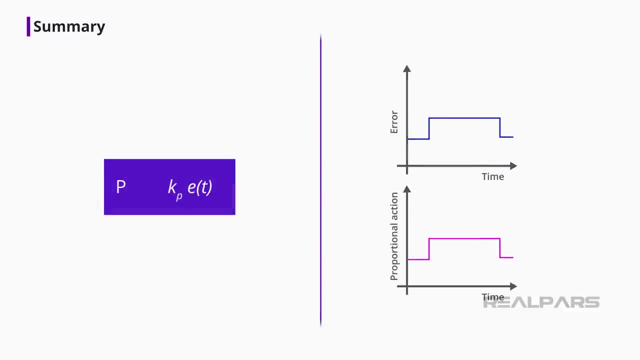 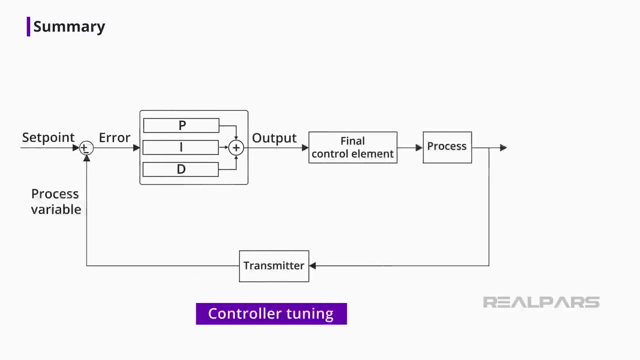 proportional to the magnitude of the error signal. The Integral block creates an output proportional to the duration and magnitude of the error signal. The Derivative block creates an output signal proportional to the rate of change of the error signal. Controller tuning involves correctly setting the controller P, I and D values. 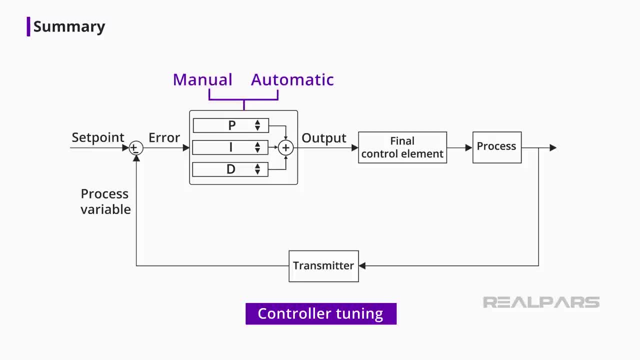 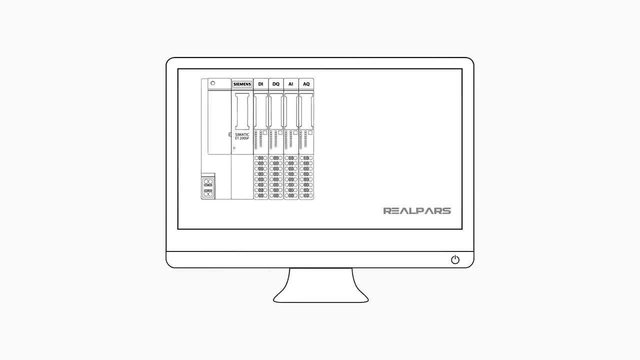 for specific process requirements, either manually or automatically. Want to learn PLC programming in an easy to understand format and take your career to the next level? Head on over to realparscom to learn more about PLC programming.